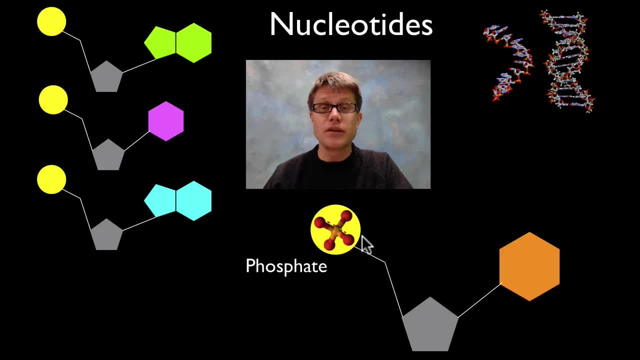 oxygen around the outside. Phosphate groups are really famous in biology, So they're the phosphates that are found in phospholipids that make the cell membranes of all life, And it's the same phosphate that we're going to find in ATP, adenosine triphosphate. It's 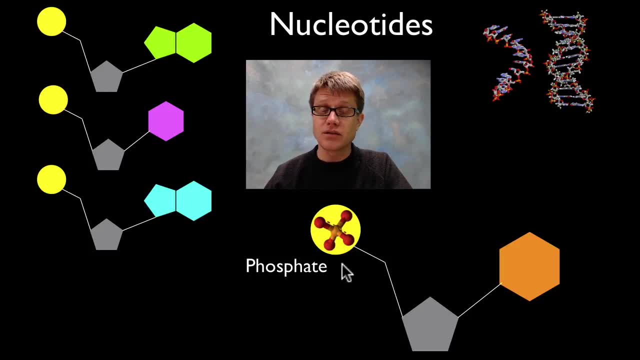 the energy source And in fact the adenosine triphosphate is exactly the same adenosine add to make DNA. We'll get to that in just a second. What else do we have? Well, we have a pentose sugar. Pentose sugar means we have a five carbon sugar In DNA. that's going to 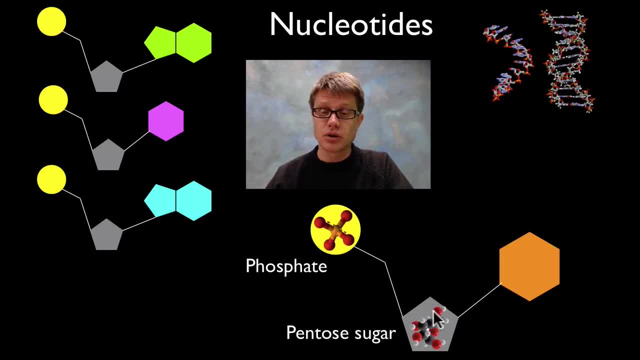 be a deoxyribose sugar And then in RNA it's going to be a ribose sugar, And then the most interesting part of a nucleotide is going to be the nitrogenous base. And it's called a nitrogenous base because it has nitrogen, And so most things in life are made up of. 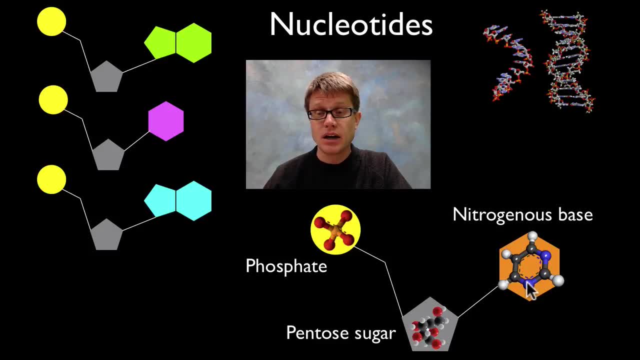 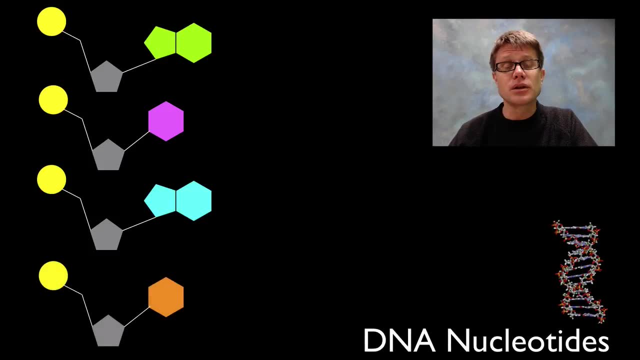 carbon, But there's going to be a lot of nitrogen here in the base of this nucleotide, And this is going to be different in each nucleotide, And so let's take a look at the nucleotides found in DNA, And so basically, you have adenine, cytosine, guanine and thymine, And so we have 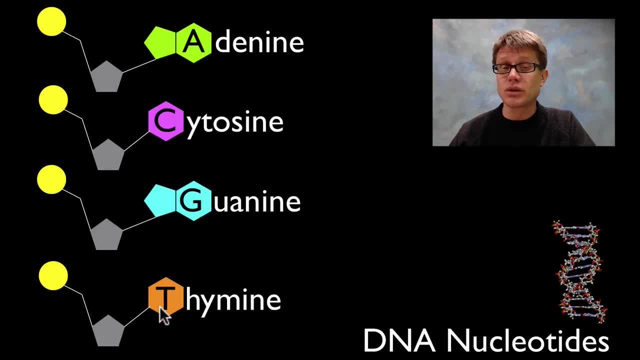 four different bases and therefore we have four different nucleotides And you can just see, looking at them, the size is going to be a little different on all four of these In RNA. they don't have thymine- You might know this- But they have uracil. It's going. 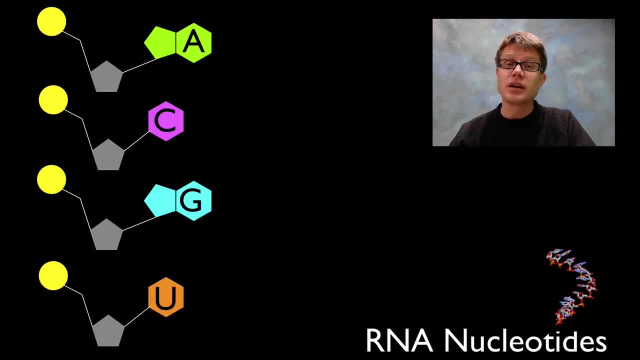 to look a lot like thymine, But it's not going to be thymine If we were to now look at all those nucleotides together, So A, C, G and T- And that's where the names come from- In DNA we're talking about these nitrogenous bases or these nucleotides. 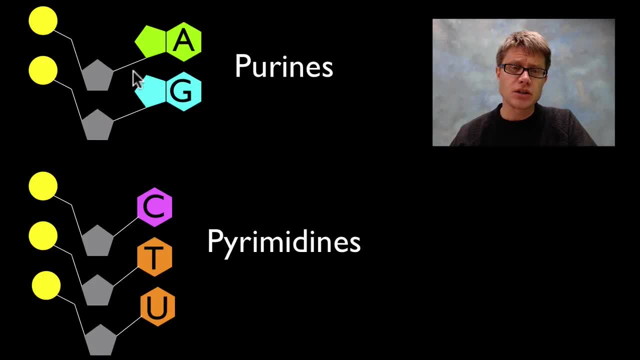 Now we've got uracil. Basically, if we put them in order by their size, we've got two major groups. We have these ones that have two rings And we call these purines. So this is adenine and this is going to be guanine. And then we have the pyrimidines And they're 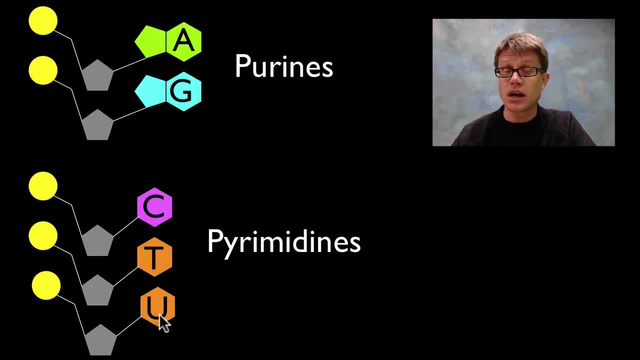 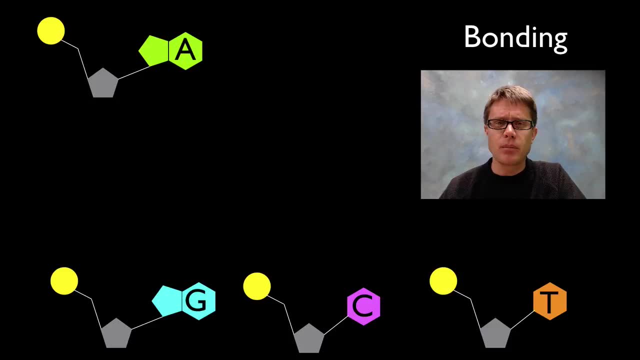 just going to have one ring. So cytosine, thymine and uracil are all going to have one ring. So they're going to be smaller, And that will become really important when we start bonding them together. So let's talk about bonding. How do you connect them together? Well, when 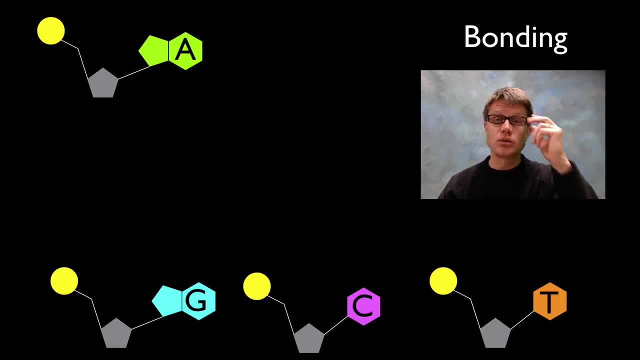 we talked about carbohydrates, there's really only one way to connect carbohydrates. Or when we talk about amino acids, there's really only one way to connect them. But, especially when we get to DNA, you can connect nucleotides in two ways. So let's start with way one. 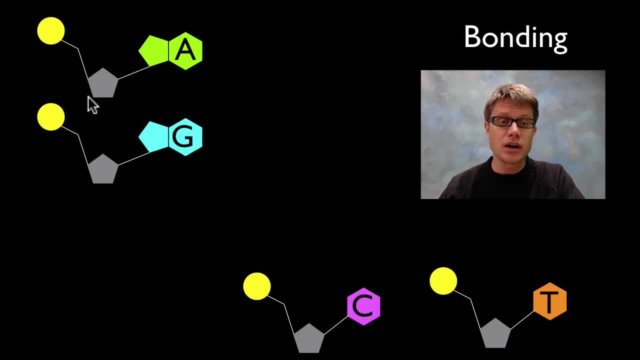 Way one, we could put this one right underneath it. So we've got an adenine and a guanine And then, through a dehydration reaction, we could lose a water right here and we could form a covalent bond between two nucleotides. And so if we were to add another one, we would add another. 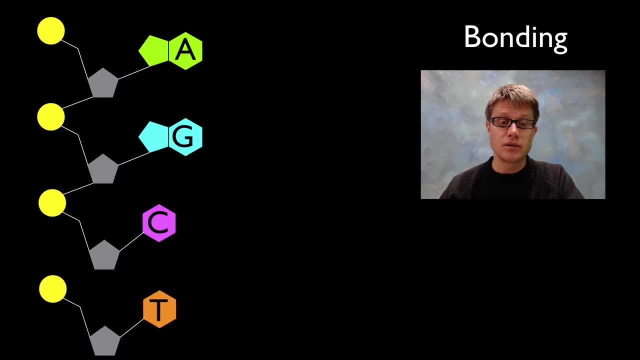 nucleotide. here We lose a water and we're going to make another covalent bond, And so we can attach them together like that. And so that's what RNA is. RNA is a number of nucleotides simply in a row, and they're connected with covalent bonds. between each one There's 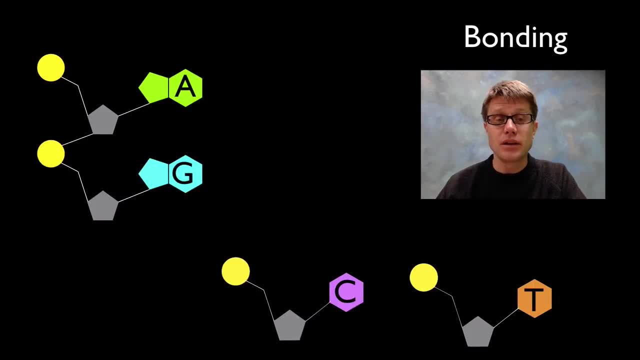 another way, however, when we get DNA that we can bond them. And so let's say we have these two nucleotides, adenine and guanine. How could I attach this thymine right here? Well, basically I can turn it upside down and it's going to form hydrogen bonds here between the adenine. 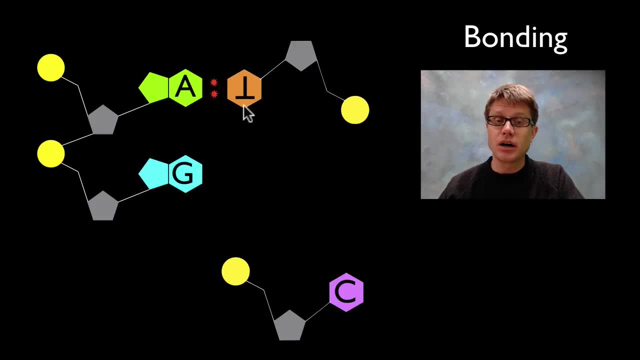 and thymine, And you've probably heard this before. The adenine will always bond to thymine and guanine will always bond to cytosine And that's why There's going to be interactions between the oxygen nitrogen and the hydrogen and make these hydrogen bonds that are going. 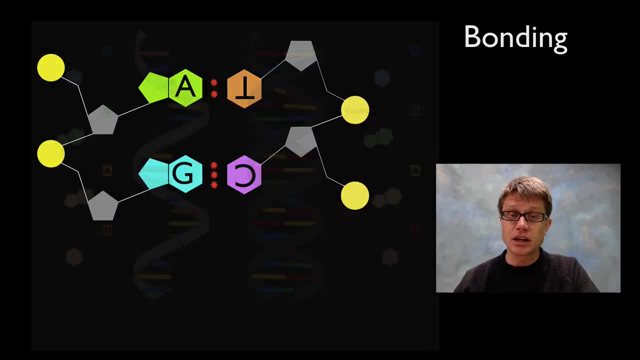 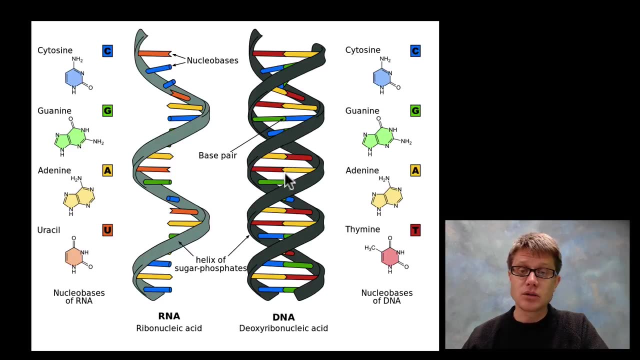 to connect the two. And so when you're looking at DNA, let's kind of switch to this next slide. When you're looking at DNA, that's what's being connected right here in the middle. So that's going to be those hydrogen bonds between the nitrogenous bases on either side. 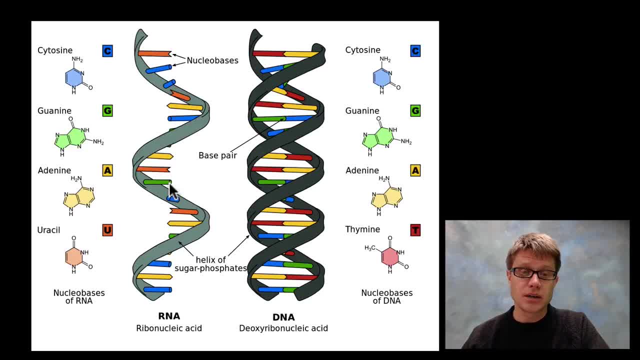 And so why do we have DNA? Well, we think life started with RNA because it contains a message. But over time we kind of had two RNAs wrap around each other and we eventually had DNA. There's more to it than that, But DNA is going to be a more stable structure. We're going 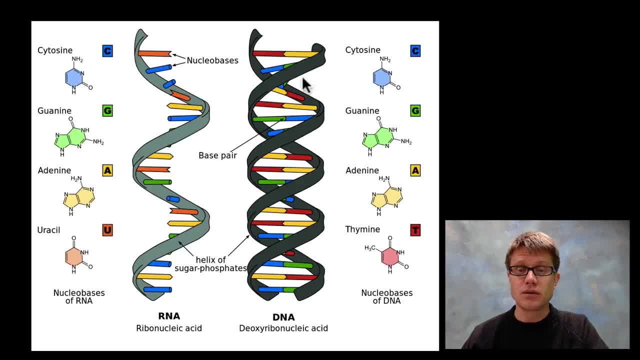 to have these hydrogen bonds here, And then we're going to have hydrogen bonds between different backbones of the DNA as well. And so what are the backbone of DNA really made up of? It's just a sugar attached to a phosphate to a sugar to a phosphate to a sugar, And 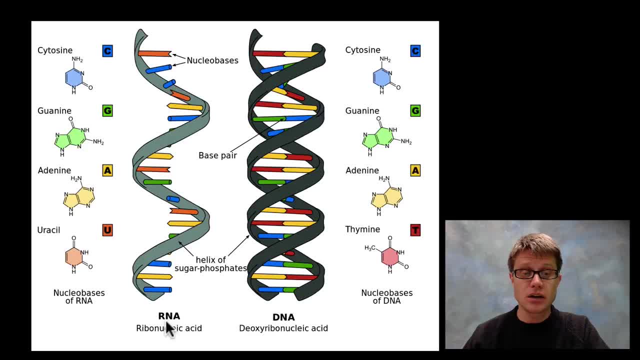 so what are some differences between DNA on the right and RNA on the left? Well, the first one would be the uracil versus the thymine, So that's going to be a different nitrogenous base. DNA is going to be a double helix And RNA is going to be a single helix. And then 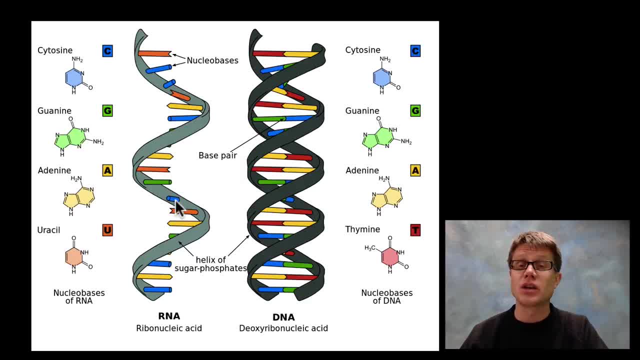 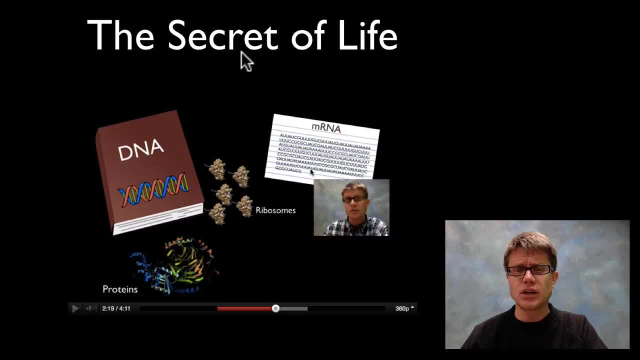 in life. DNA is going to be found in the nucleus And RNA is going to be found pretty much everywhere that we need it. So if you're confused on how we go from DNA to proteins, or if you're really interested in the whole secret of life, you're going to want to look at this slide. 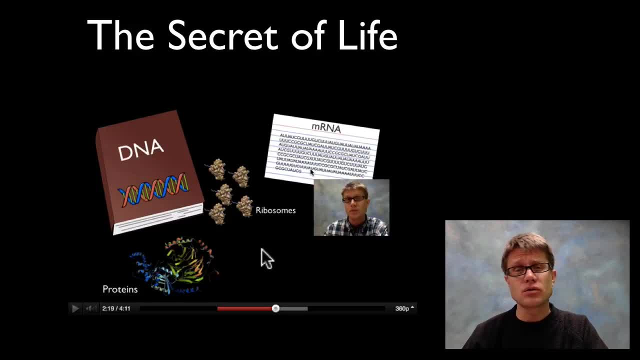 I'll put a little link to a video I made that kind of talks you through how we go from DNA to proteins. But the last thing I wanted to leave you with is how important they are. If you're interested in RNA and if you're interested in science and video games, then 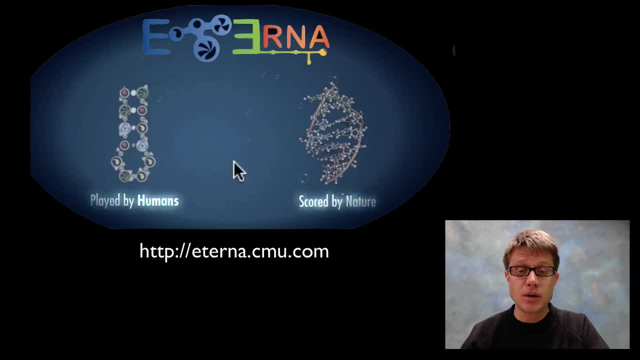 you may want to check this out. This is Eterna. Eterna is a video game, I think it's centered at Stanford University And basically what they're doing is they're letting people on the internet build sections of RNA And so, basically, you build sections of RNA. They 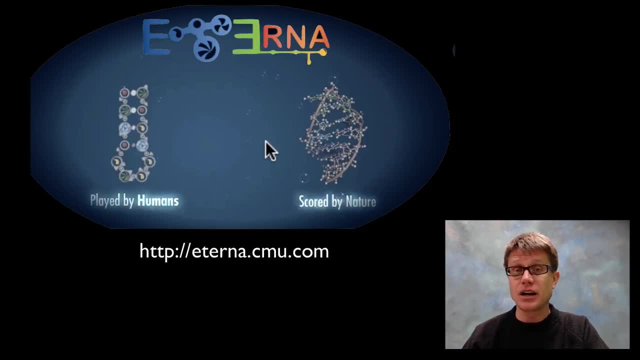 build sections of RNA each week And basically the winners- each week they will make your RNA. So they'll actually synthesize and make your section of RNA And then they'll see how it does. And so I'm going to launch the video game and talk you through the first. 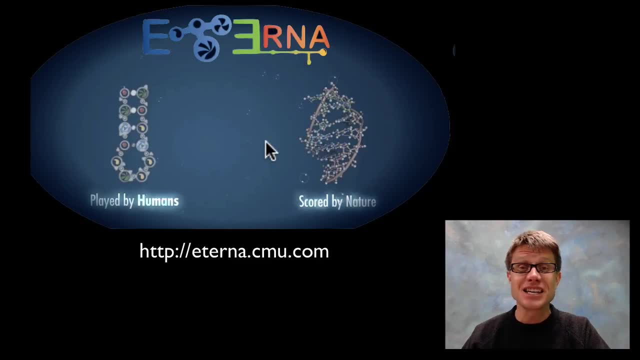 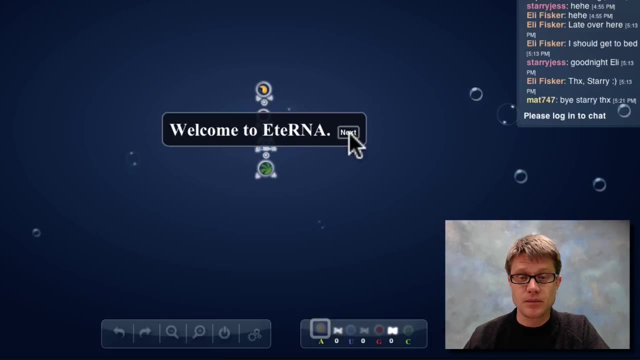 level, And if you're interested in RNA or making things real in biochemistry, you may want to give this a shot. Okay, So here is level one. Basically it's a tutorial, So I can click on next and it will talk me through what I'm going to do. So you're going to build. 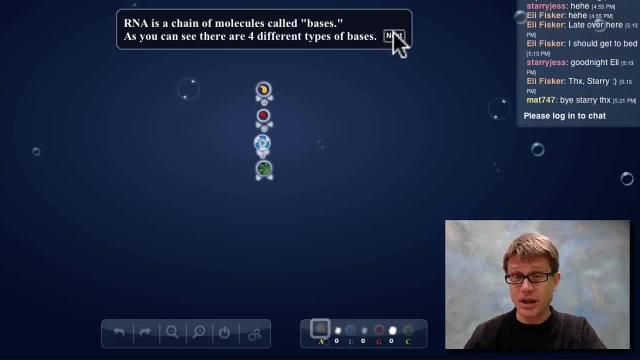 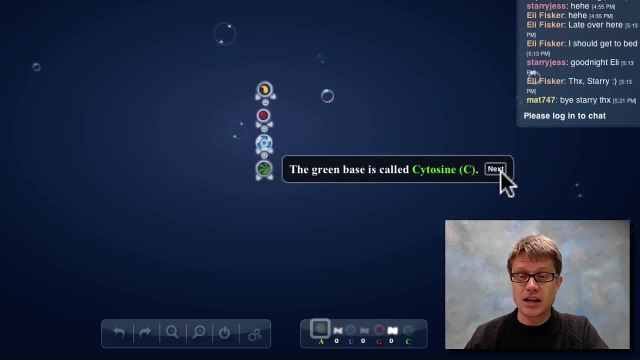 your own RNA. Let me click on the next one. RNA is made up of four bases. Hopefully you'll know what that means now. The yellow base is adenine, guanine, uracil and cytosine, And so, as a warmup drill, let's convert all the bases to guanine. So let me click here. 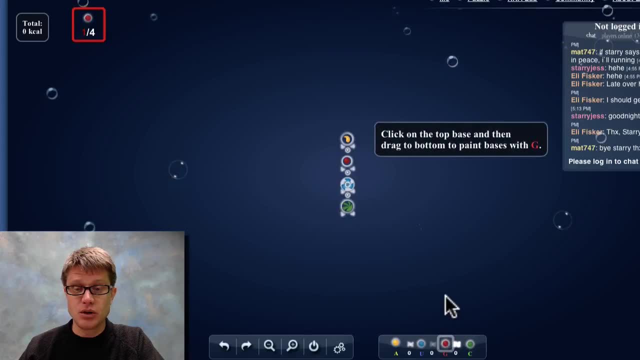 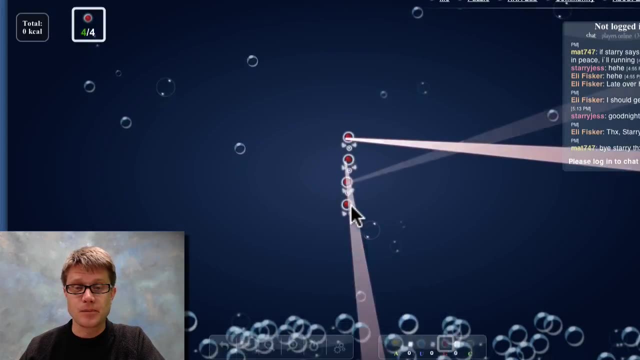 to start. So basically what you can do is go down here I'm going to get my mutate And I'm going to mutate this to guanine. I love the music in here, the little sound effects, Nice. So I cleared level one And then you can go to the next puzzle And we can just 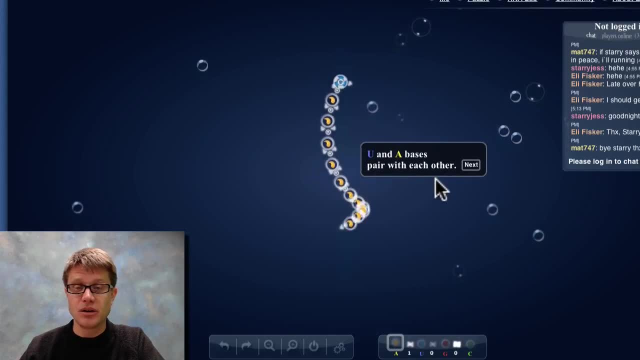 go through. And so, basically, on this one, what you can do is they will attract each other. So, for example, they're going to say that adenine and uracil are going to come together And the guanine and cytosine are going to come together, And so, basically, what you do is: 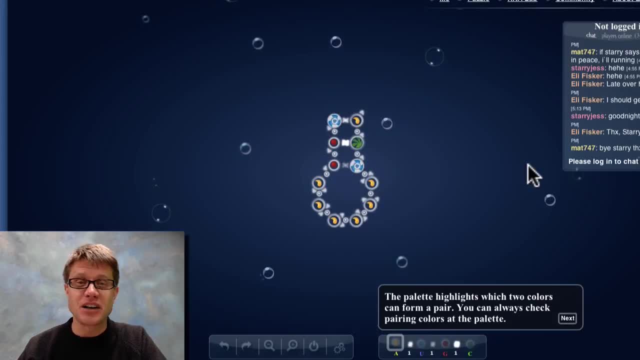 you get to play around with pairing these, And so I'm going to stop playing the video game in front of you. But give it a look. It's a really cool idea: People competing to make RNA And then they're actually building it in the real world, And so that's nucleic.